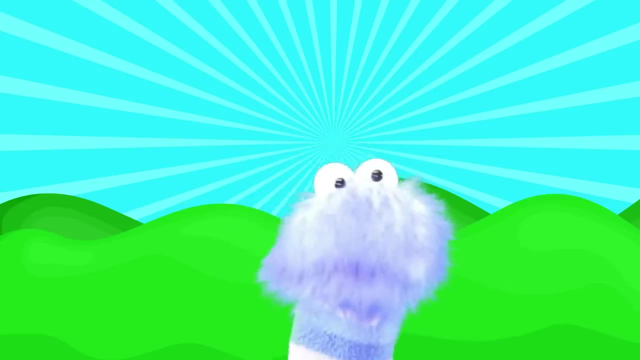 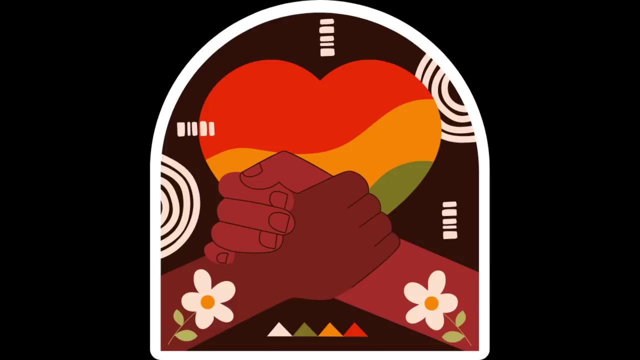 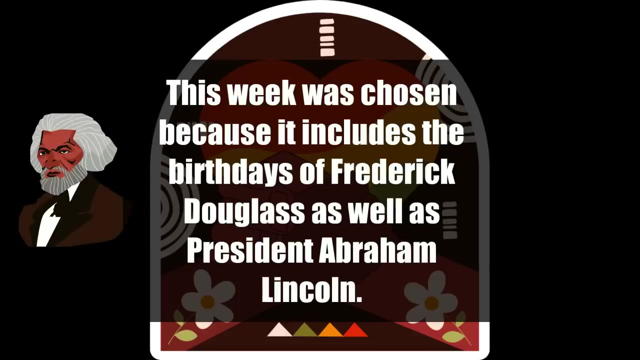 But this was not just any random week chosen in February. We're going to find out why. That's right, Gus. This week in February was chosen because it includes the birthdays of Frederick Douglass, who was an abolitionist, which is somebody who wanted to end the practice of enslaving people, as well as the President, Abraham Lincoln. 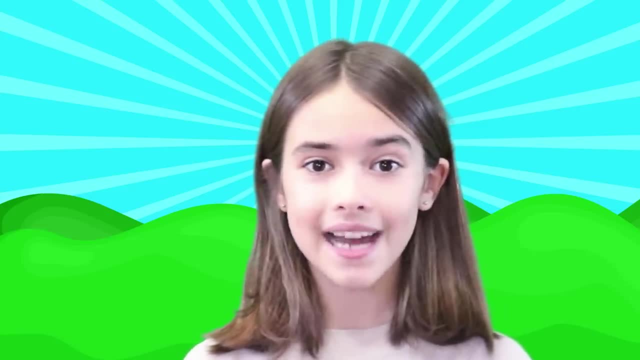 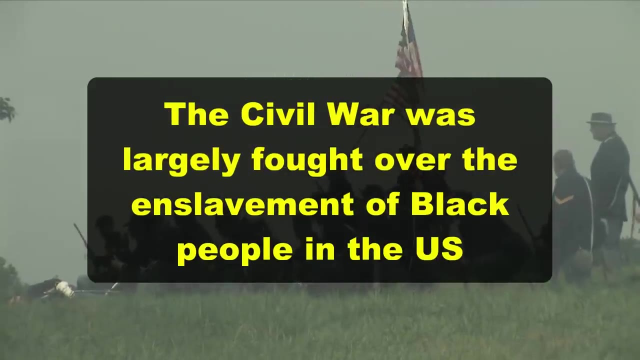 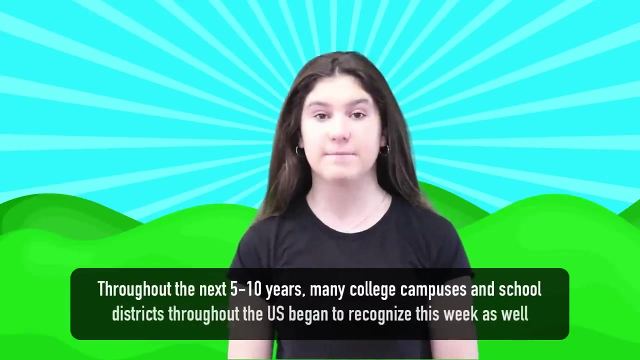 President Lincoln led the United States during the Civil War. The Civil War was largely fought over the enslavement of black people in the United States Throughout the next five to ten years. many college campuses and school districts throughout the United States began to recognize this week as well. 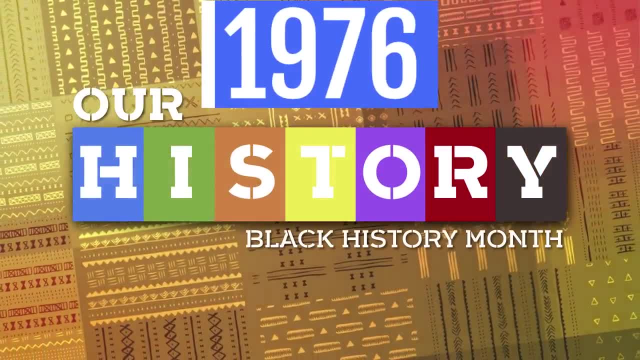 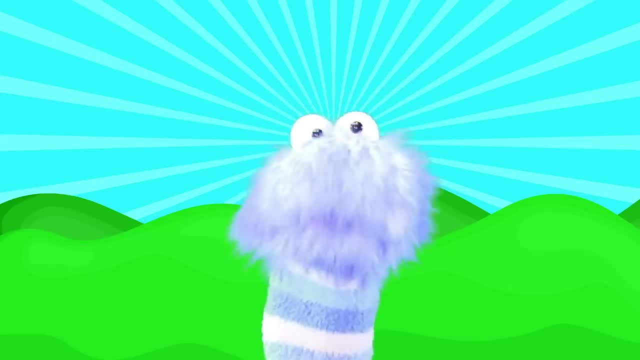 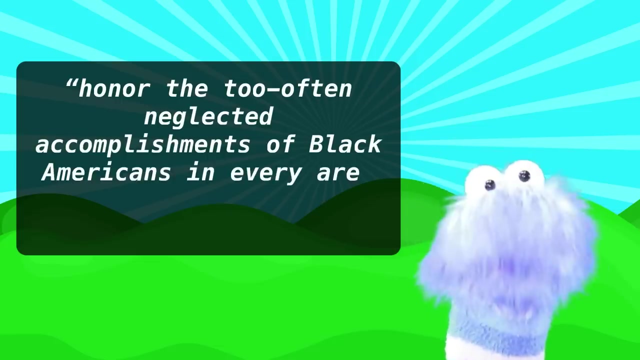 And then, in 1976, the week-long event officially became known as Black History Month. It was actually President Gerald Ford who changed the celebration to the entire month of February to, and I quote, honor the too-often-neglected accomplishments of black Americans in every area of endeavor throughout our history. 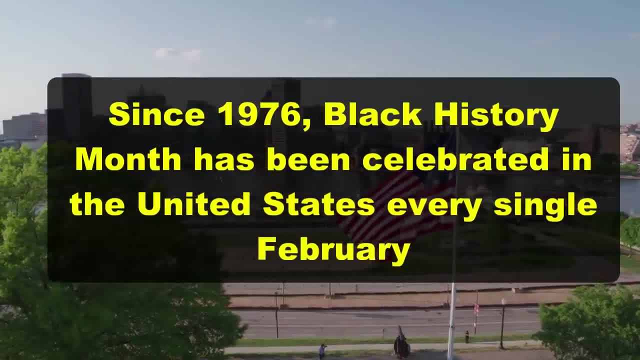 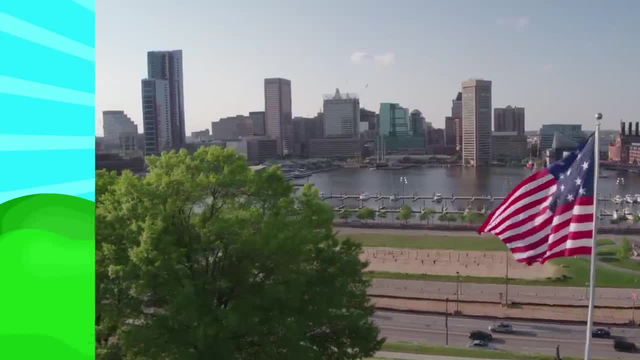 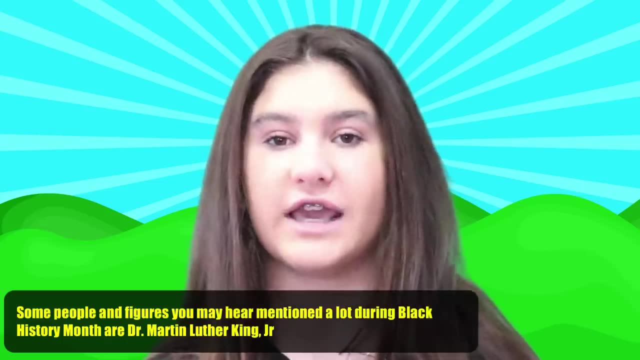 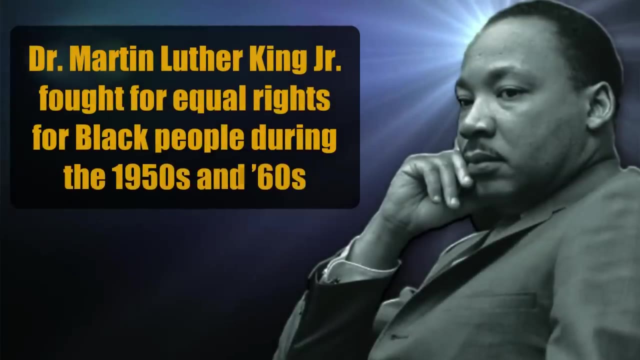 And since the year 1976, Black History Month has been celebrated in the United States every single month of February. Some people and figures you may hear mentioned a lot during Black History Month are Dr Martin Luther King Jr. Dr Martin Luther King Jr fought for equal rights for black people during the 1950s and the 1960s. 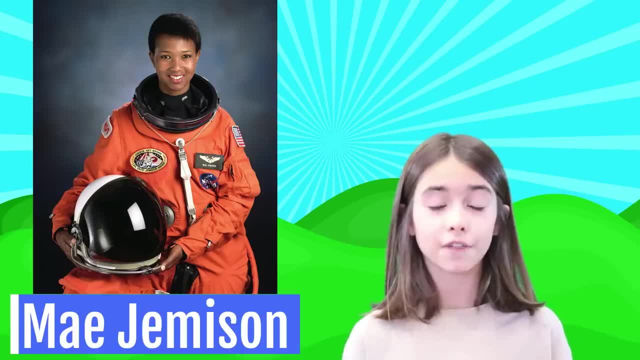 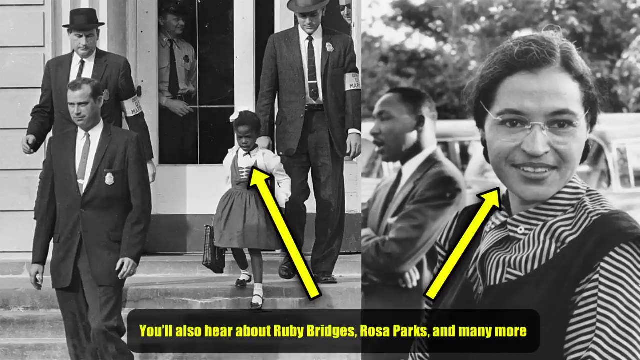 Another is Mae Jemison. She was the first female African American astronaut to travel to space in the year of 1992.. You'll also hear about Ruby Bridges, Rosa Parks and many more, And, believe it or not, we have a lot of videos about those people as well. 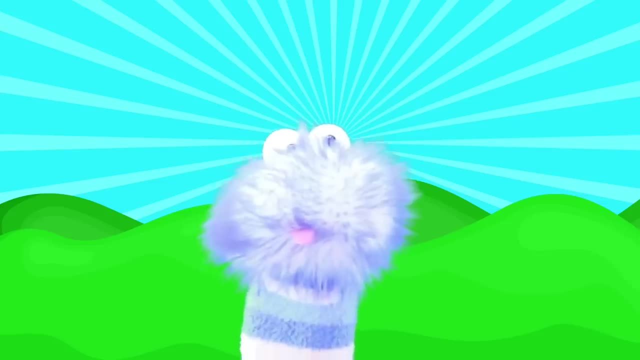 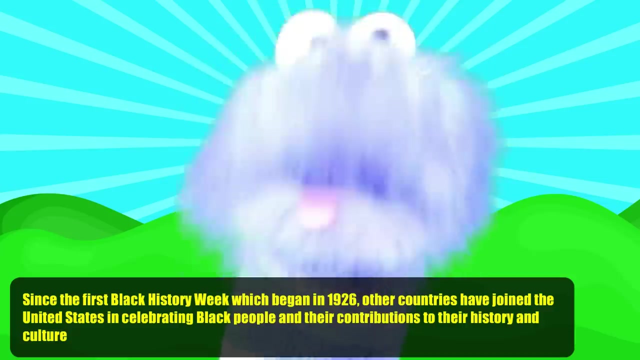 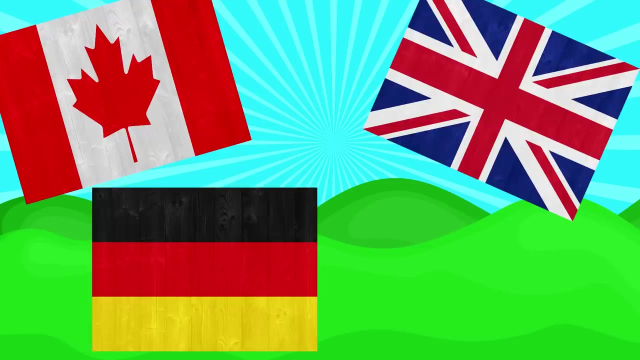 Those will be linked in the description too. Since the first Black History Week, which began in 1926, other countries have joined the United States in celebrating black people and their contributions to their history and culture, And these countries include Canada, the United Kingdom, Germany and the Netherlands.